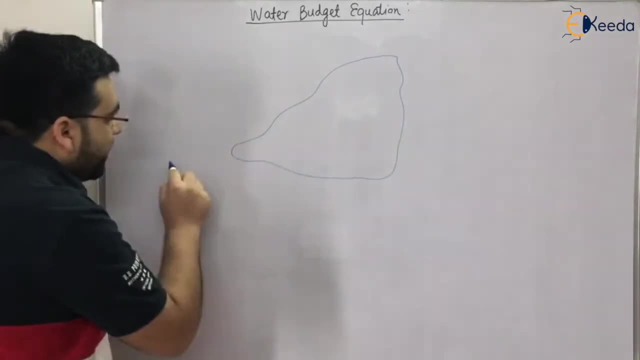 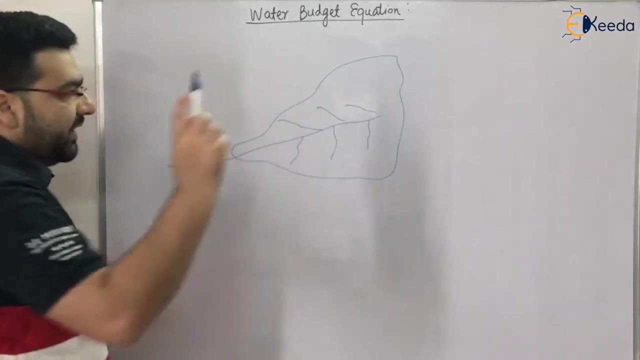 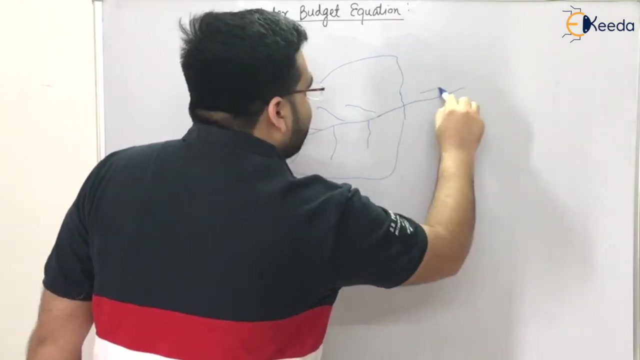 area- let me understand, let me make you understand- is the catchment area. this is the river, these are the tributaries. let us say that these are tributaries. okay, let us say this is a catchment area and we, it has some. you can say: and this is going out, this river is going out this. 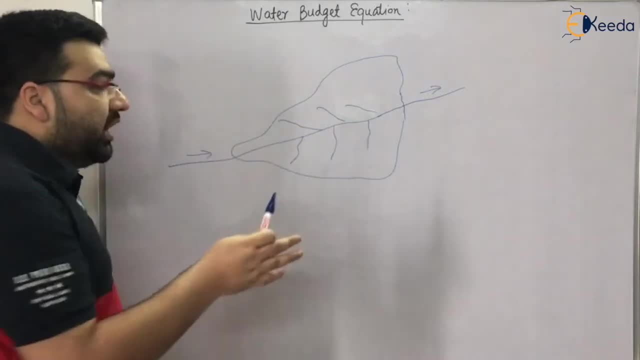 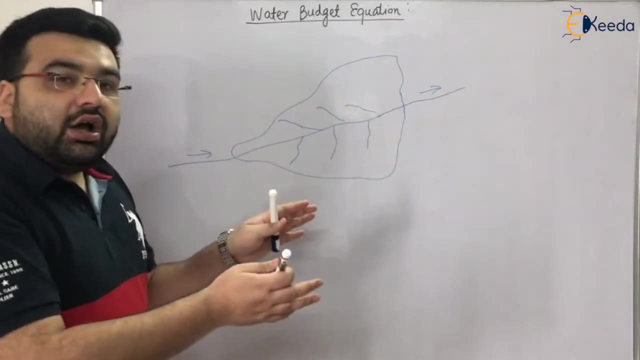 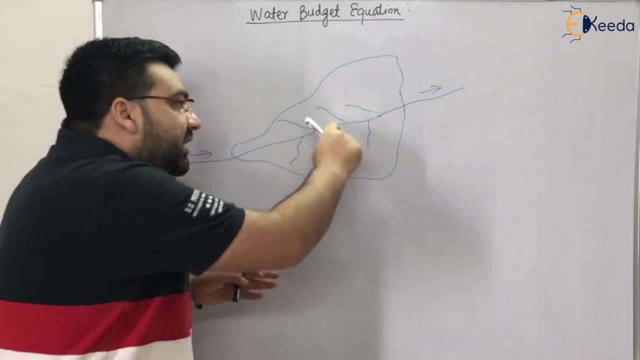 river is coming from here and going from there. this is a catchment area. now, what is a catchment area? this is very important because a lot of people fail to understand. the catchment area is the area which will contribute. again, I am repeating: the catchment area is the area which will contribute in increasing the 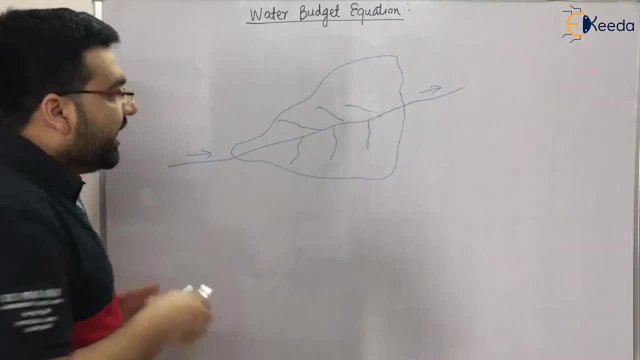 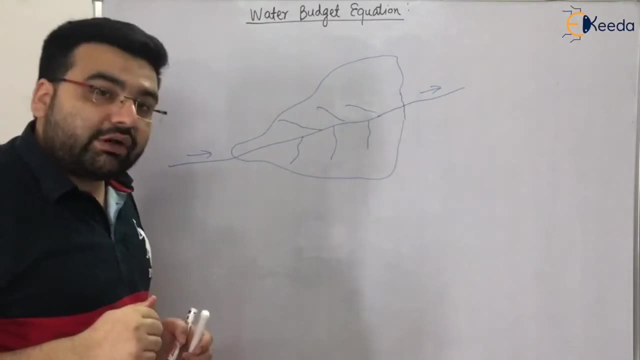 discharge of this river. okay, it means that, if I am taking this area into consideration, if rain will fall on this area, precipitation will fall on this area. what will happen then? some infiltration will be there, some transpiration will be there. evapotranspiration will be there, but some. 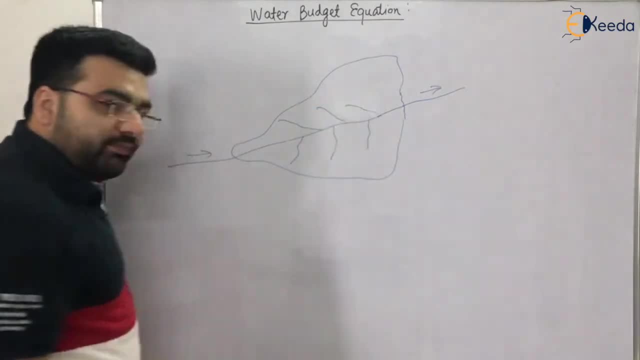 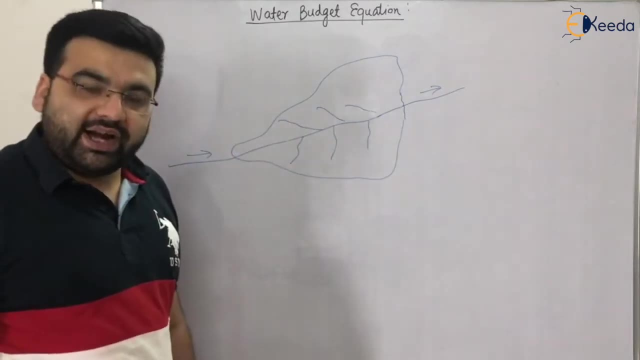 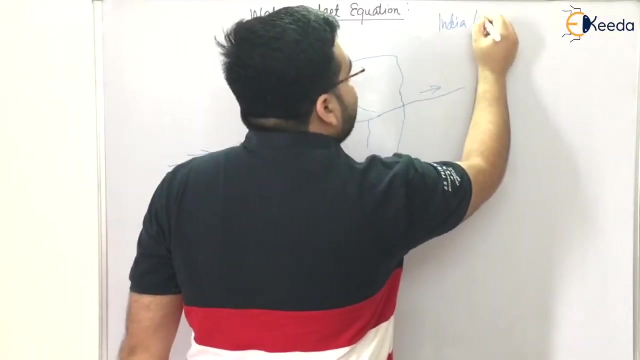 water will go to this stream here and that area which will contribute to the discharge or the volume of this stream, is known as a catchment area right. in USA it is also known as watershed right catchment area in India and British India and in British Britain. 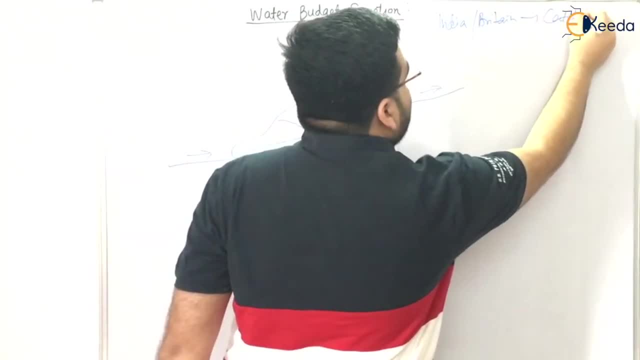 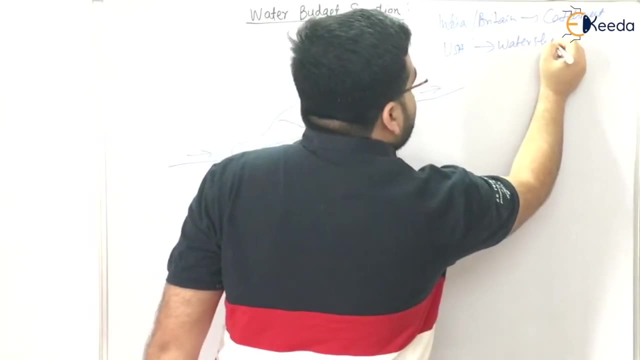 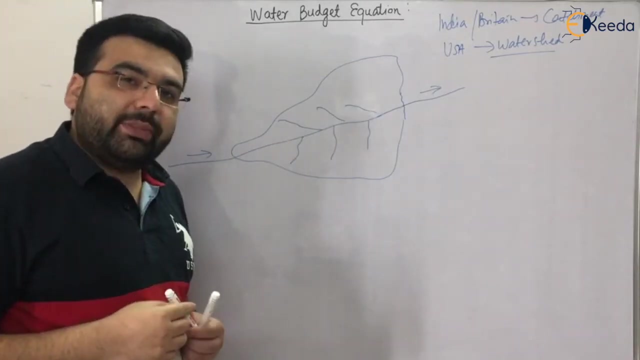 it is known as catchment, and in the USA this area is known as watershed, water shed. you must have heard about the subject watershed management right. when I was in Britain it was an elective subject: watershed management. yeah, okay, so this area is known as catchment or watershed. right now, let us say that some. 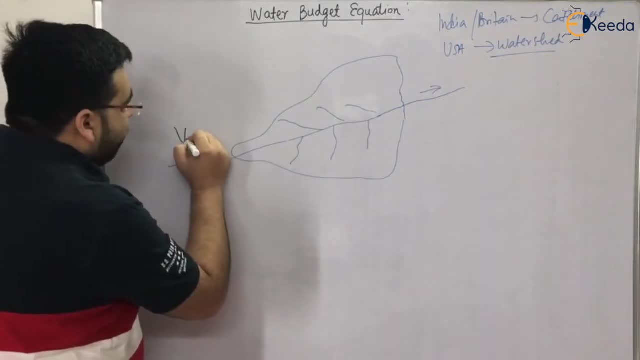 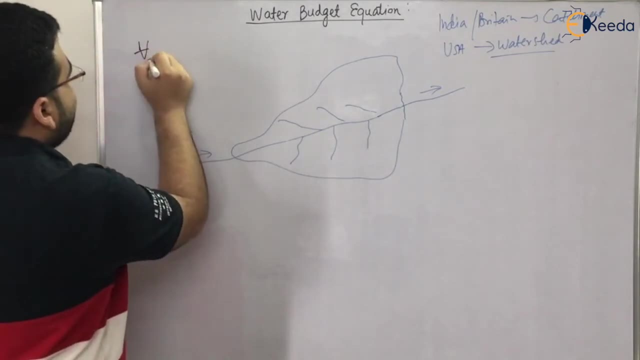 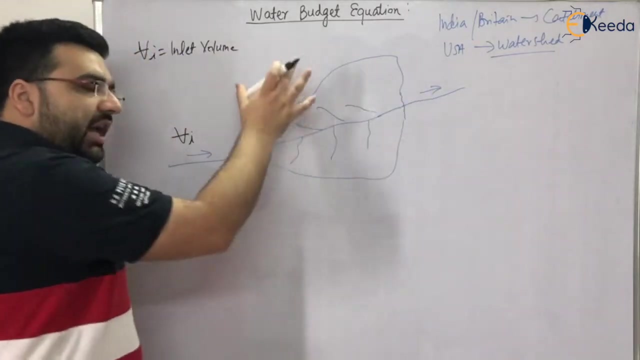 volume of water is coming. let us say that some volume of water is coming, VI. let us say this, VI clear. let VI. VI is the inlet volume, right, VI is the inlet volume, inlet volume. and let us say that after each, after something will be happening: some evapotranspiration. 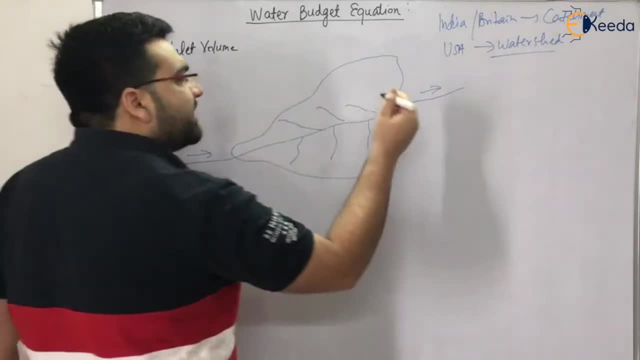 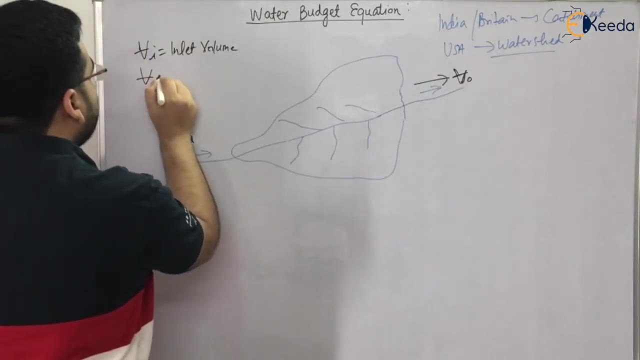 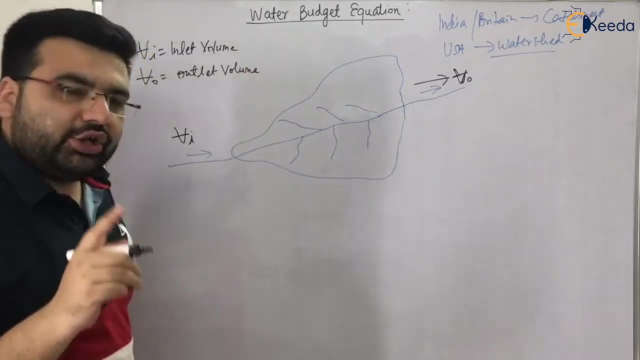 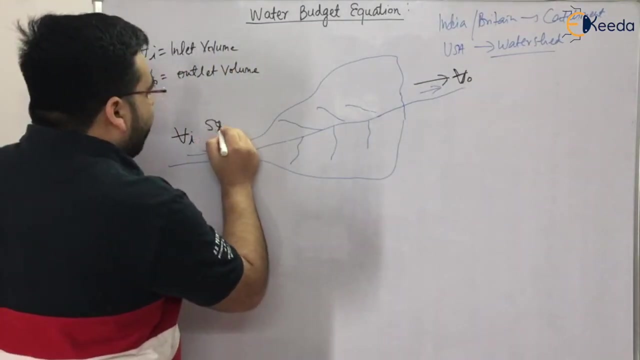 will be happening. some infiltration, some runoff will be there and after some time, let us say that this is VO out volume. right now, VO is outlet volume, outlet volume. now what a you think? you tell me, what do you think will this? VI will be equal to VO. suppose that 50 meter cube volume of water is coming from this side? 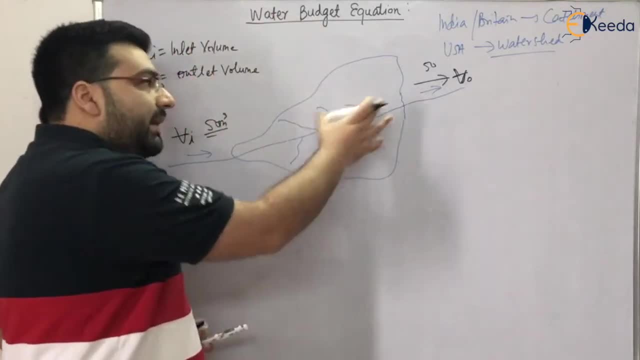 will it be 50 or this is more than 50? it can change. it can be less than 50 or more than 50. also, if there is a lot of precipitation it will be more than 50, but why? because there will be some infiltration also infilt cerca, transpiration, right. some runoff will go to the ground water also, right V not suppose that 50, because it can also change. 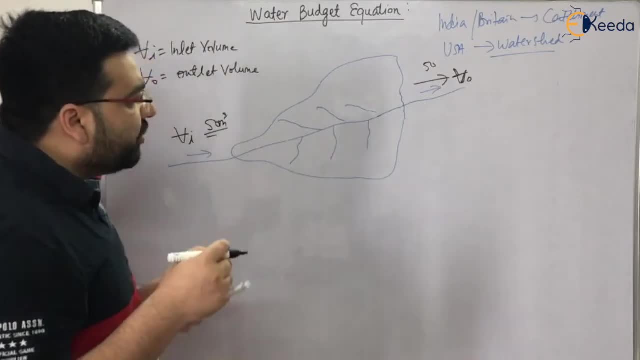 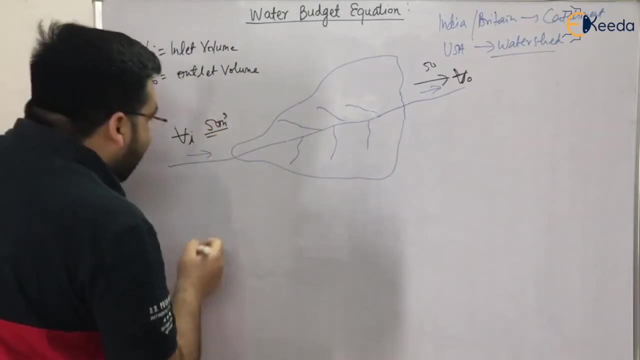 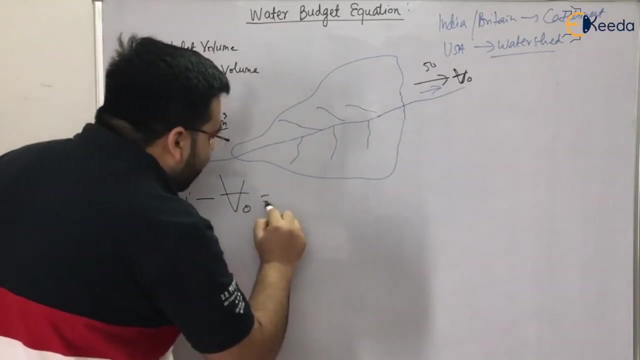 because of infiltration also. infiltration, evaporation, another transpiration, right or no? we, we adversely go to the ground water also. they have some water that is going on, you right, it can change, right. okay, so I can say that if I subtract these two quantities, that is the inlet minus outlet water, whatever the volume, I will. 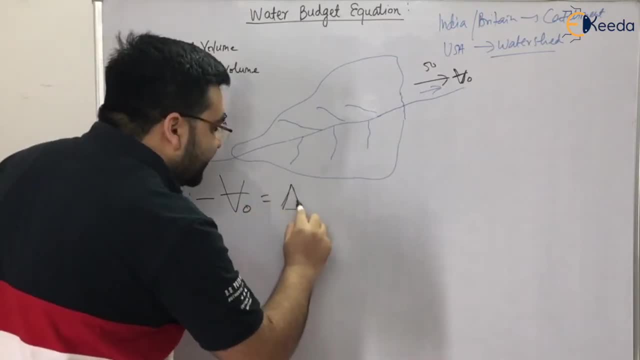 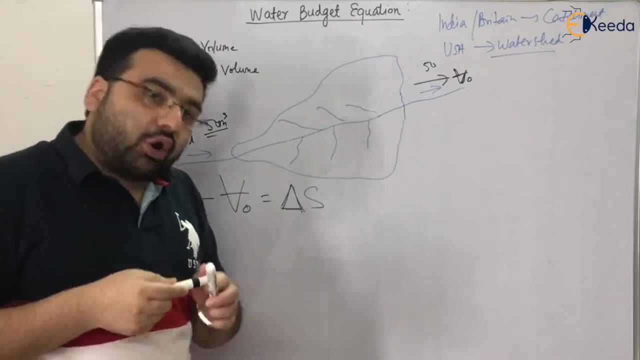 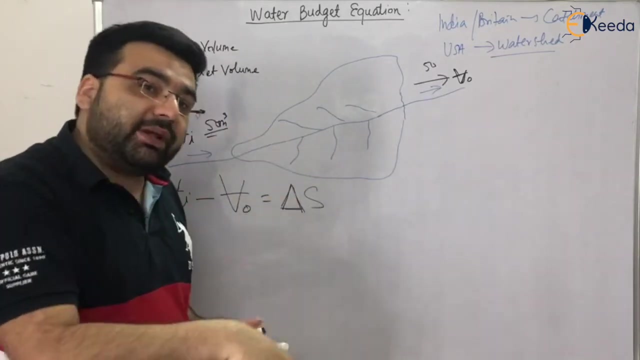 be getting. that will be storage, Delta s storage. storage means this catchment has stored that water. it can either be in the form of groundwater, it can either be in the form of. you can say there can be some depressions in this catchment area, but the water can be the depressions right or the water can be. let us say, 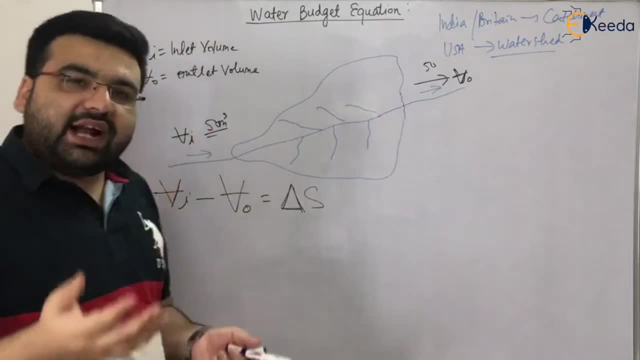 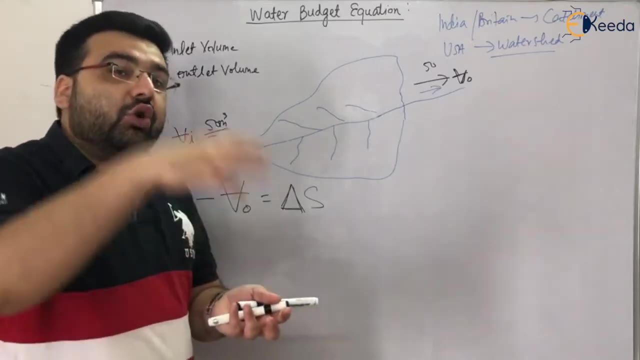 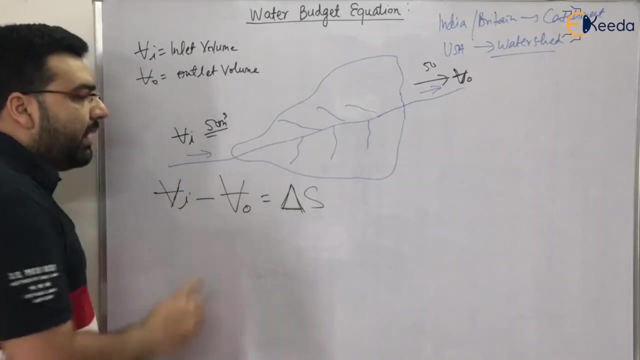 that time of pond is there or some other thing is there. it can be that also I, or if suppose that the plants also, they also carry some water on them right, which they do not transpire. okay, that water will also contribute to storage. so I can say that the mass inflow minus the mass outflow is the change in storage. but 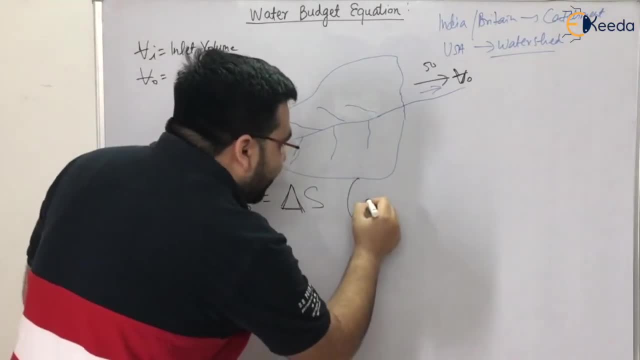 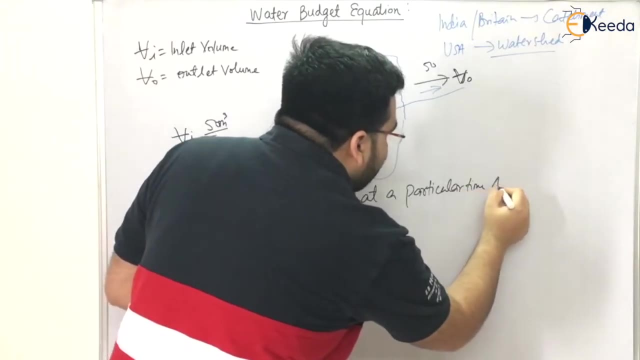 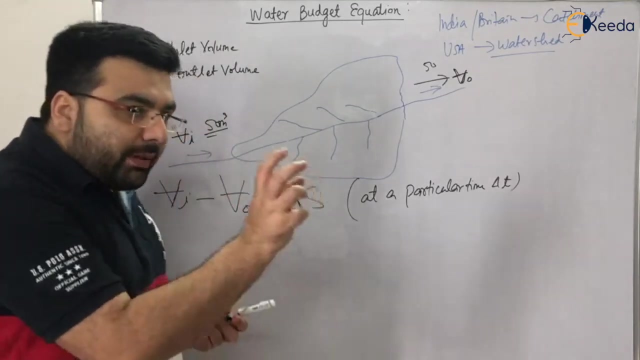 remember one important thing: this is at a particular time T at a particular time del T. this is for a particular time. it can be at 2 pm, 3 pm or 4 pm. right, there should be a particular time frame interval for both. 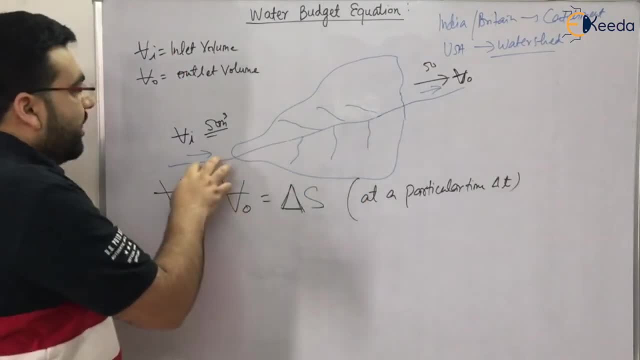 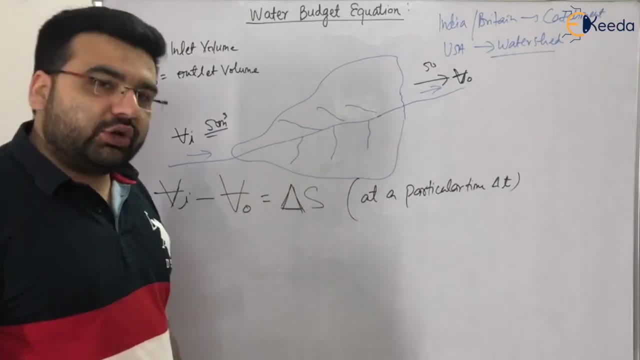 inflow and well as well as outflow. it should not feel like that you are measuring your inflow at 5 pm and you're measuring outflow at 7 or 8 pm, right it? there should be a particular same time interval for those things. 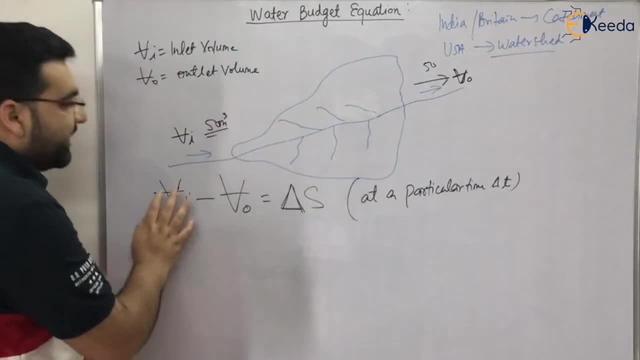 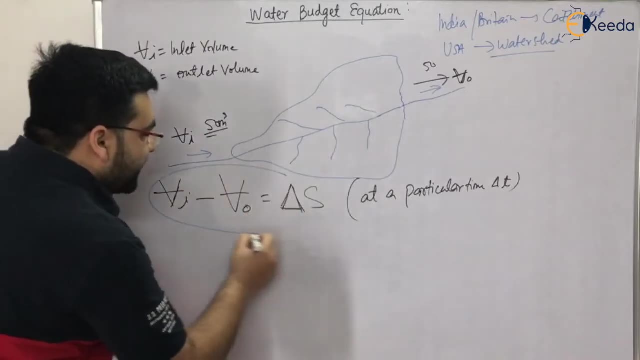 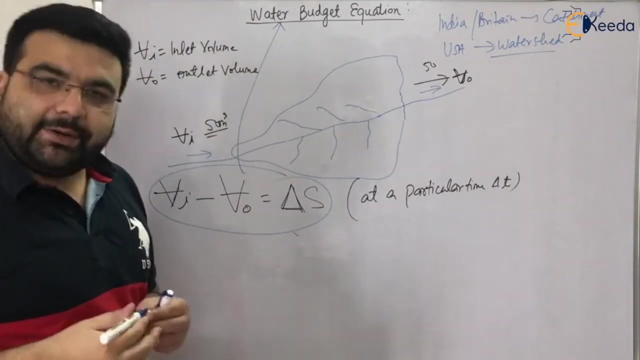 right. so for at a particular time interval, del T, the mass inflow, the mass flow, will be equal to the change in storage. and this equation is a very easy question. this equation is known as the water budget equation. this equation is known as water budget equation for a particular catch material. I hope you. 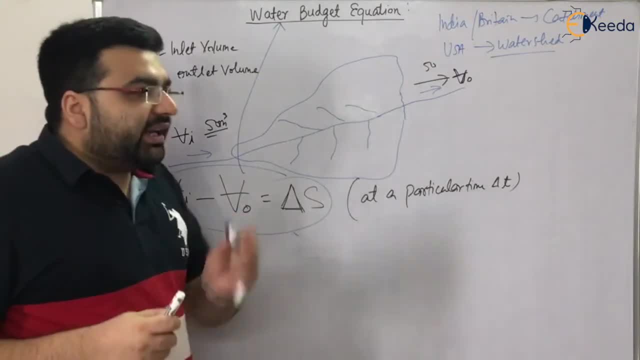 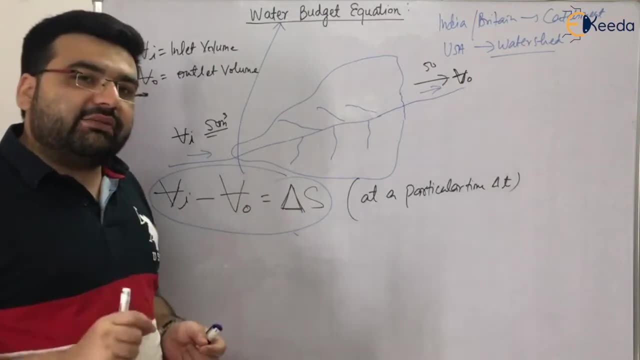 have understood now. sometimes the numericals are coming in depth. sometimes it is not given to you. it is not given to you that is 10 meter cube or 15 meter cube. some depth is given to you. so I would like to tell you that whenever we are, 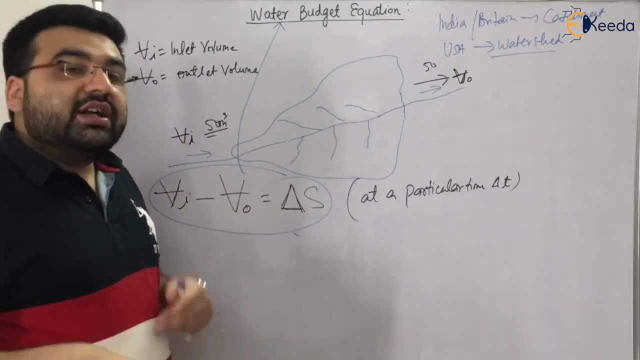 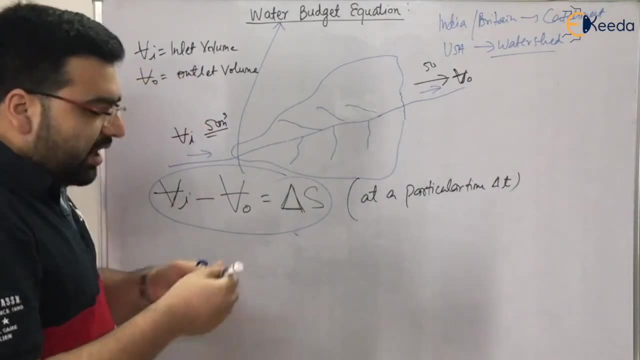 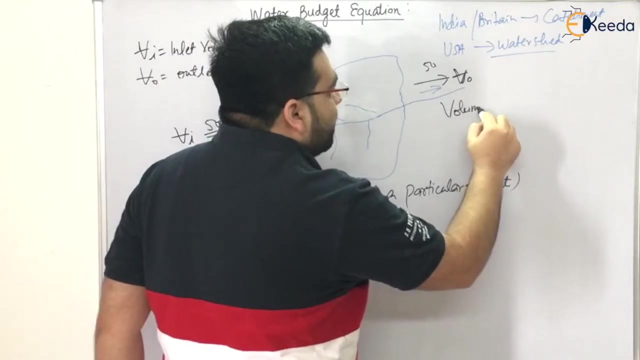 dealing with the hydrology, whenever we are dealing with the hydrology, sometimes what we do, that instead of volume will represent as depth, for example, let me give an example. let us say that. I give an example. let us say that the volume of water, the volume of water is, let us say, a 15 meter cube. let us say it is not 15. 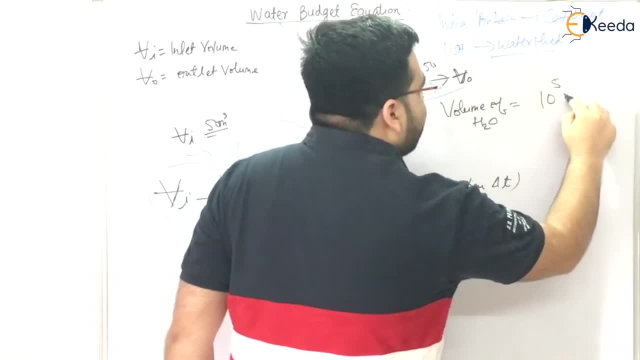 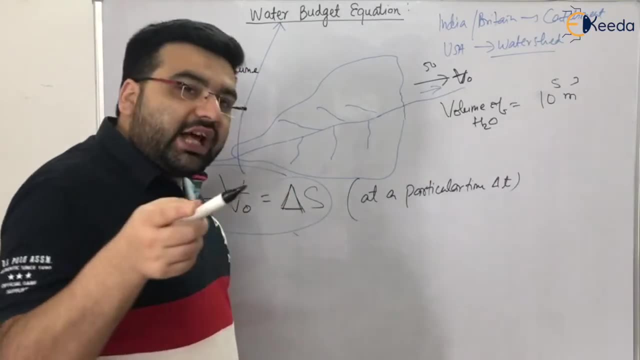 let us say it is equals to 10 raised to the power 5 meter cube. let us see the volume of water. your particular catchment is 10 raised to the power 5 meter cube. and now your what is the area of that catchment? because if in hydrology you dont know that area, 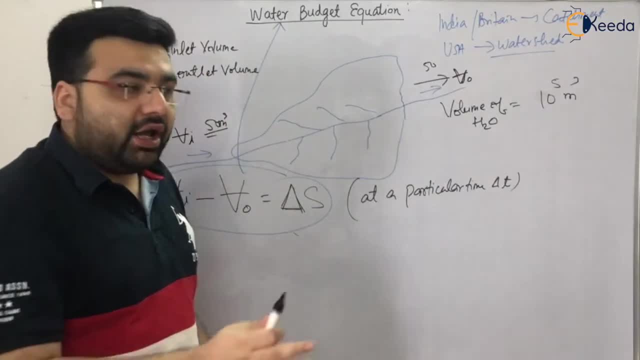 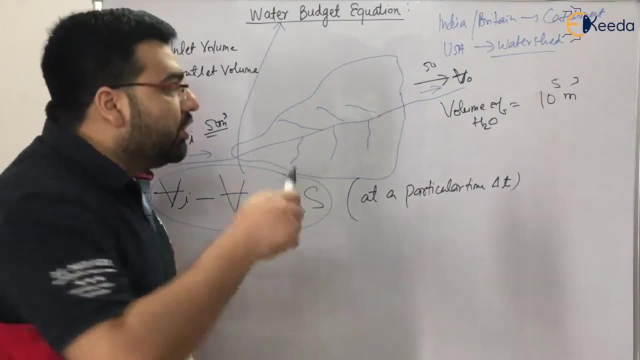 you are incomplete, right. so to have to be a hundred percent complete, you must know area of the catchment also right same the both with irrigation also right. so area of catchment must be known. so now you, you tell me, sir, the area of the catchment. we measured it with plain limiter and 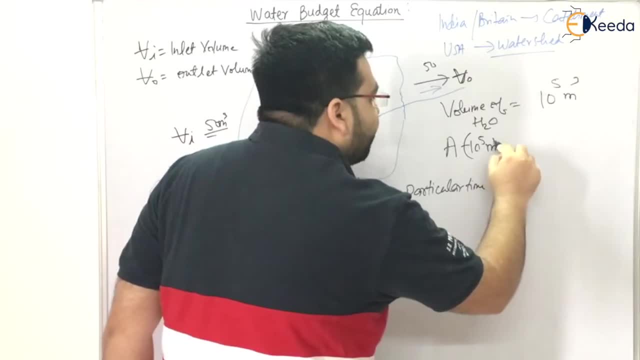 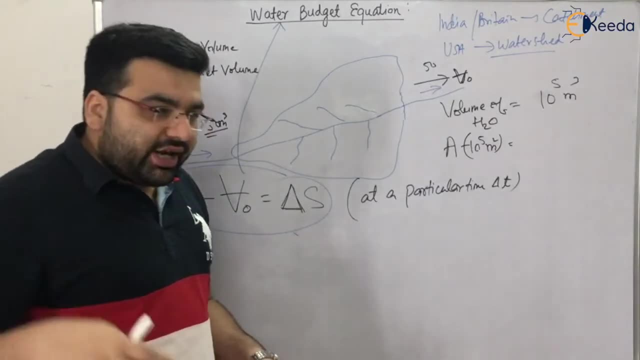 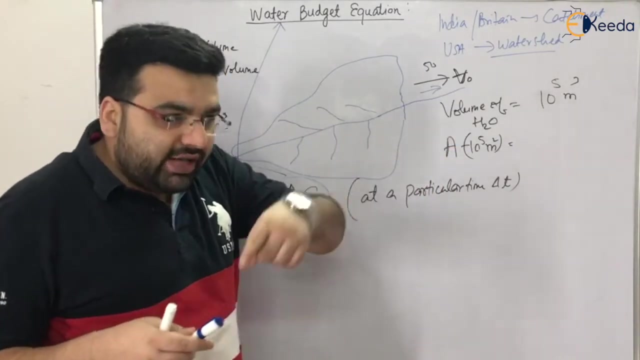 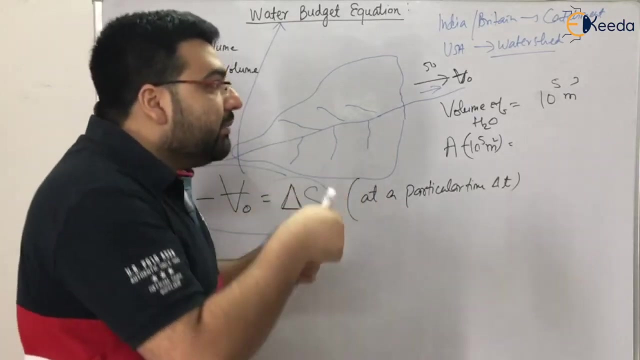 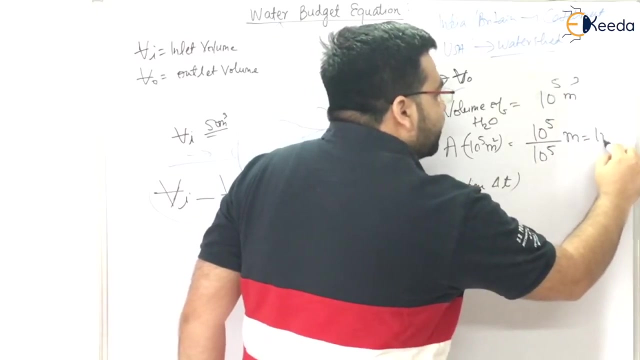 some other instruments, It came out to be again 10 raise to the power 5 meter square. Now just apply some mind. If 10 raised to the power 5 meter cube of volume of water is in area of 10 raised to the power 5 meter square, there will be some depth of water also, because volume is equal to length into width, which you have already got, as the area into height also. So there will be some depth of water right Now, what will be that depth of water? It will be equal to 10 raised to the power 5, divided by 10 raised to the power 5.. It will be meter, that is, 1 meter, or I can say 100 centimeter. 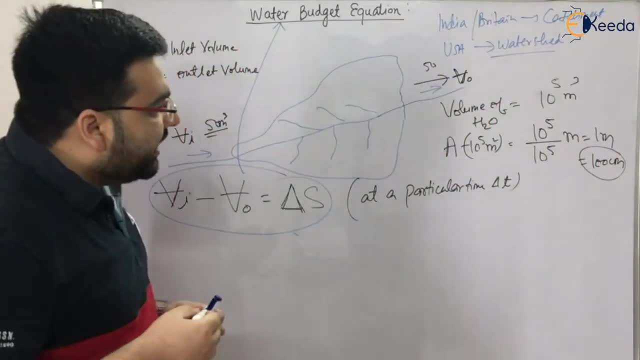 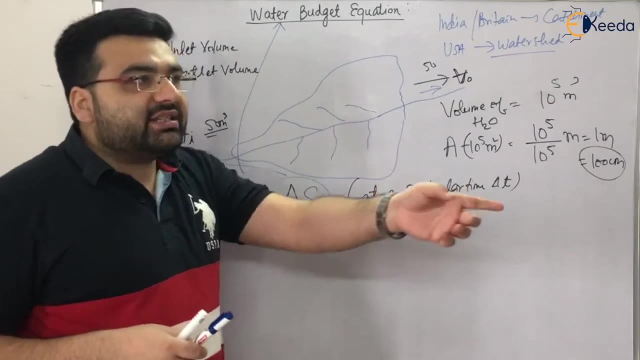 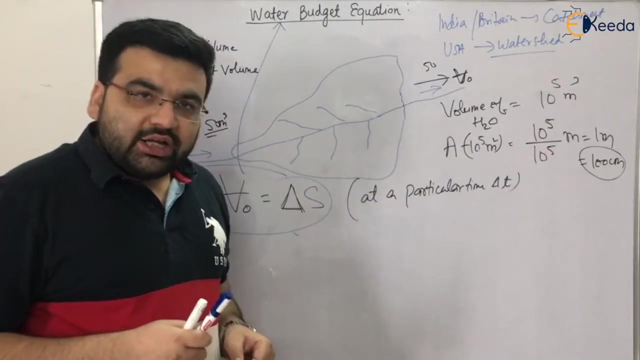 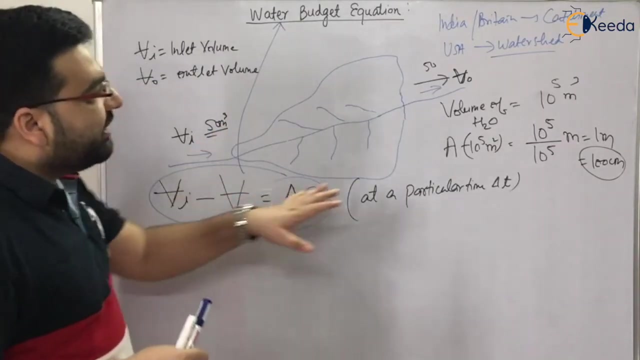 Now you will say me that, sir, in an area of 10 raised to the power, 5 meter square, the depth of water was 100 centimeter. Then I will understand. Okay, It means that the volume of water would be 100 into 10 raised to the power 5 meter cube. Right? So I hope you have understood. If in numericals, I will solve in numerical also. If in numericals, instead of volume, you are given depth, Then what you have to do, You have to calculate the volume, because this is in volume. 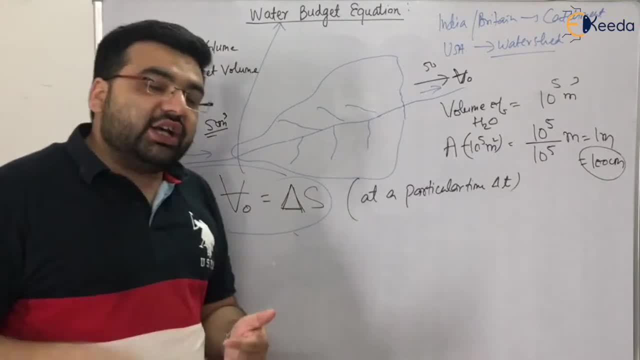 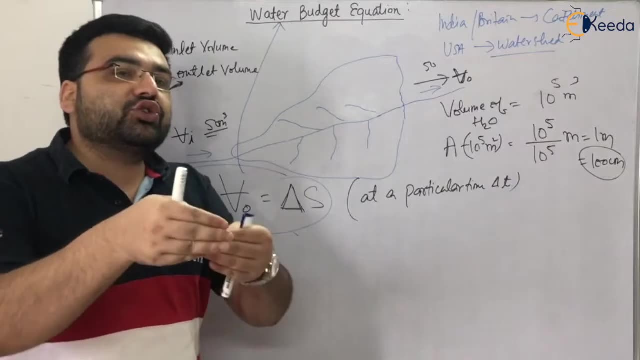 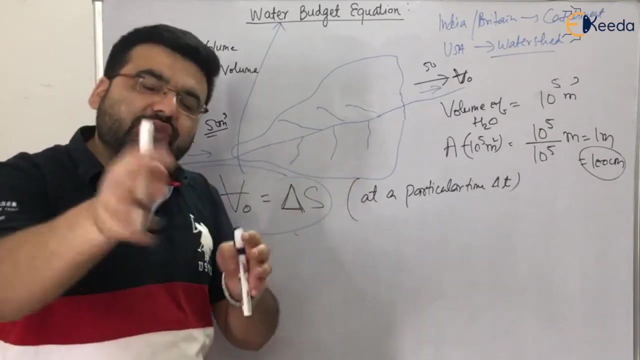 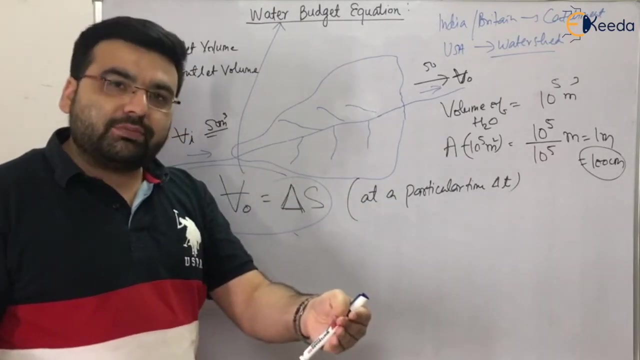 Right. The second thing is that suppose in question discharge is given to you Now you know that. again in hydrology also we frequently make use of units Right In irrigation. also, suppose that you are stuck with some numerical. just check the units, you will get the answer. Even in environment, also in activated sludge process, in your oxidation pond process, a lot of numericals are there. Even if you are stuck somewhere, just compare the units, you will get the answer. 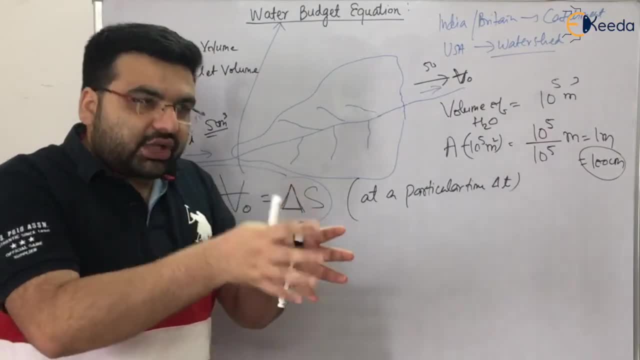 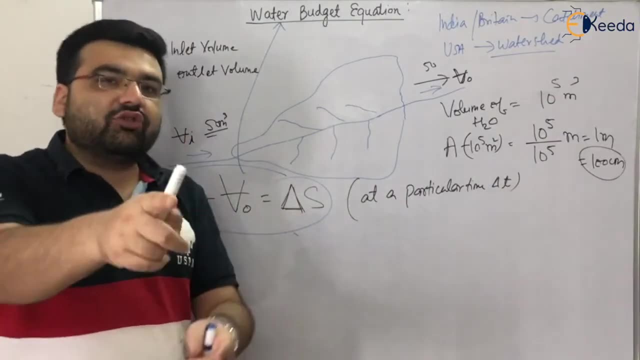 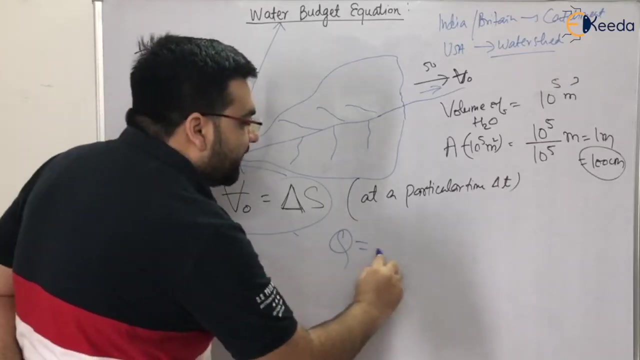 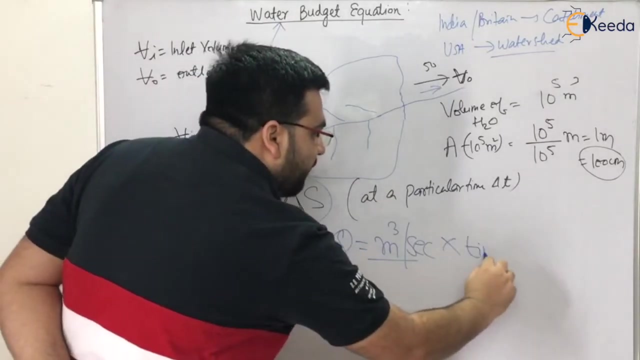 Right. It has happened with me a lot of times that I got stuck somewhere in the numerical. I compared the units, I got the answer. Similarly here also: if you get stuck somewhere, compare the units, you will get the answer Right Now. for example, if in question, it is given to you, discharge is given to you. What is the unit of discharge, Meter cube per second? Cumec, Right? If you multiply your discharge with time, what will you get? You will get volume. You will get volume. 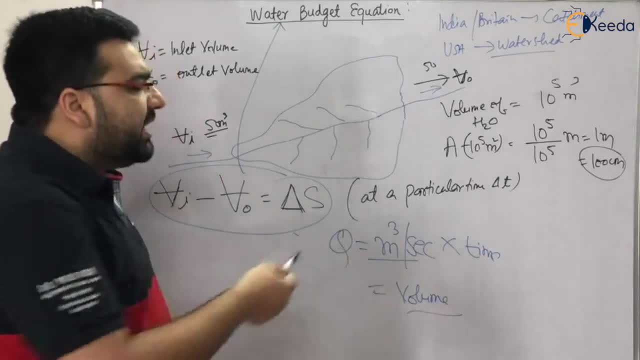 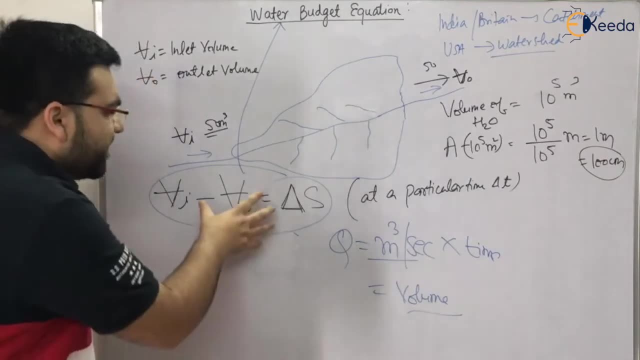 So suppose, if discharge is given to you, What you have to do? You have to multiply your discharge with time so that to get the connected volume Correct volume Clear. But the water budget equation is this only Right? No need to worry at all. Now let me expand this water budget equation. 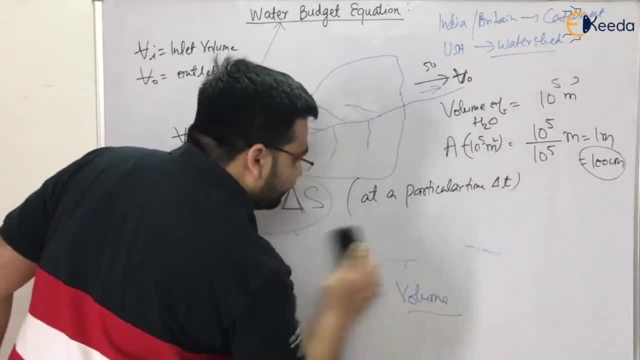 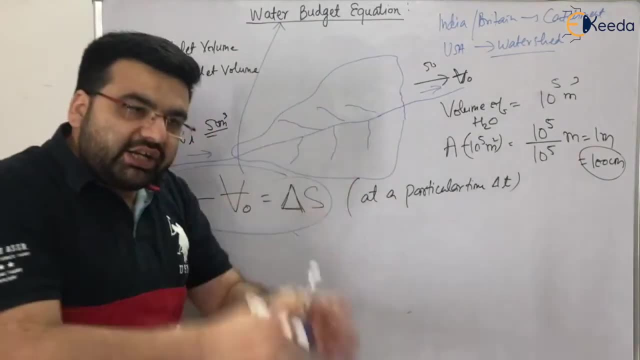 Now let me expand the water budget equation, Let me rub this. The water budget equation can be like this, also For this particular cache material: what is the inflow? What is the inflow? If there is rain, there will be some inflow, Right? 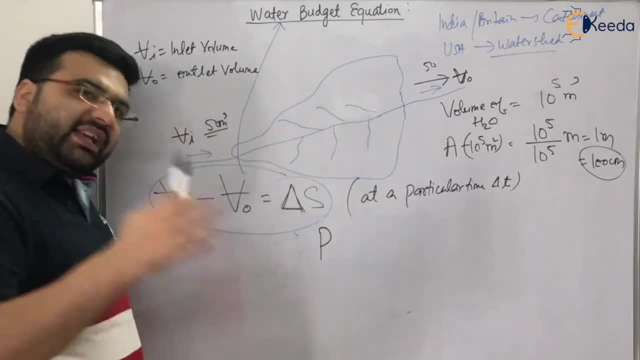 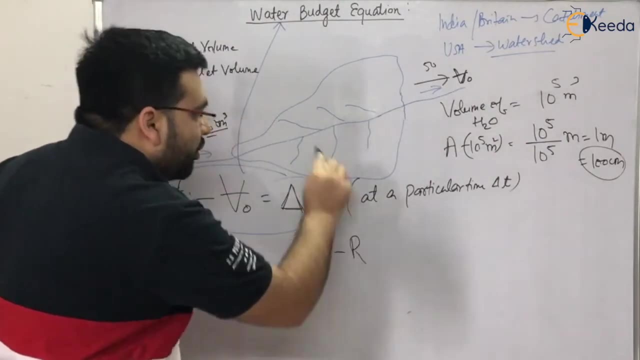 rain I denoted with the precipitation P. P is the inflow now, inflow is P now. what will be the outflow now? there will be some runoff. some runoff will be going to the outflow, right, or what can happen? just think. think there can be some. 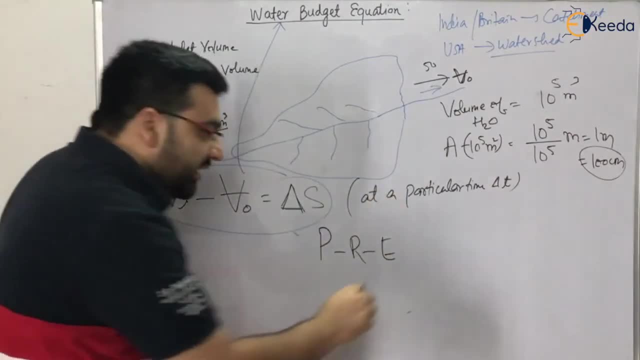 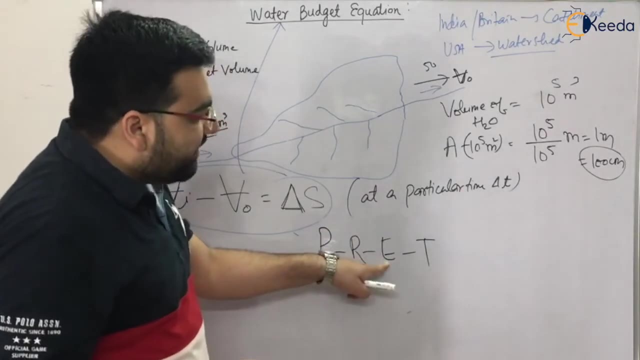 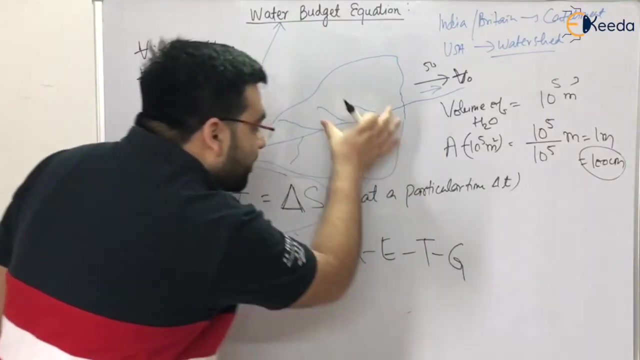 evaporation also. there can be some transpiration also. what is evaporation? what is transpiration? what is the difference between the two? when I will explain you about the evapotranspiration in the subsequent topics I'll be explaining in detail. right, there can be some groundwater, also some water. 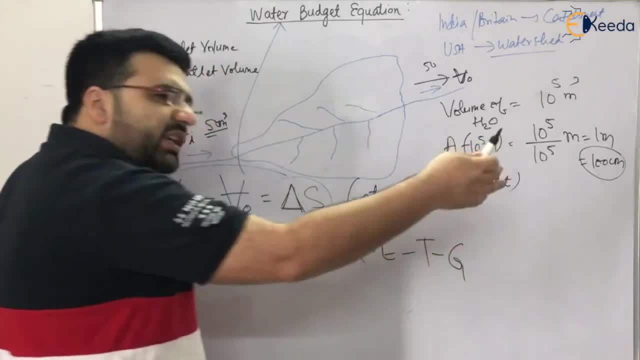 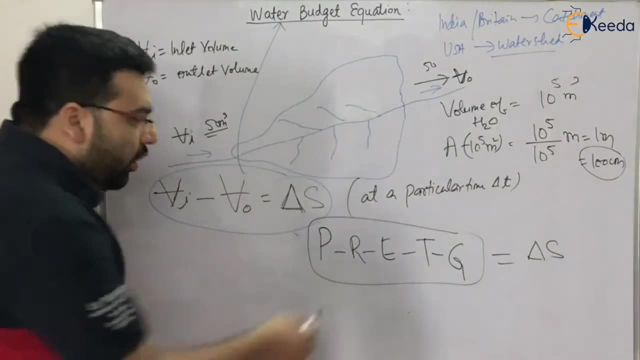 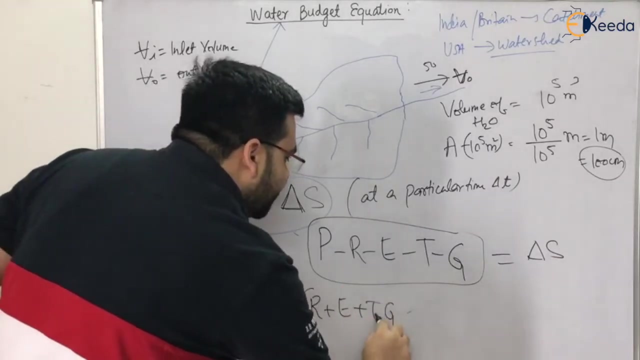 may be percolated into the groundwater also right, and other things also. but broadly, these four, these five things, right, it will be equal to Delta S. change in storage, simple. or I can also write like this: P, take minus common R, plus E, plus T plus G is equal to Delta S. so this is a detailed water budget equation. 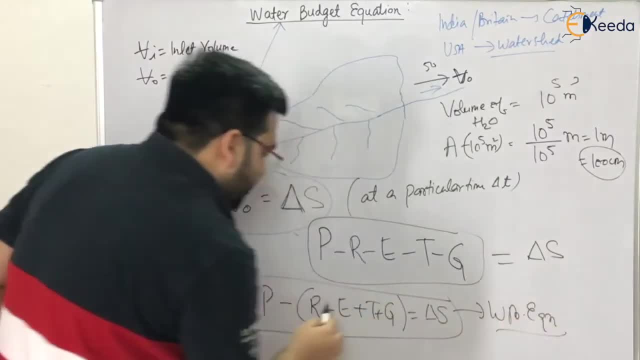 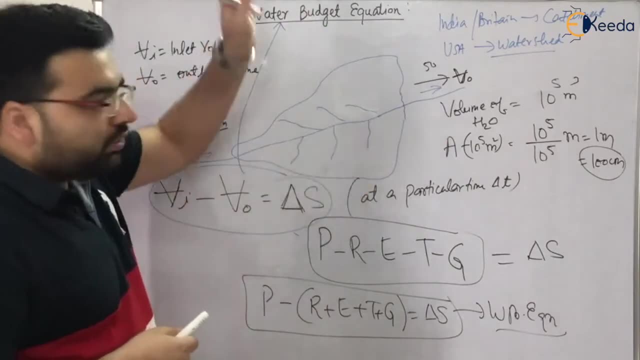 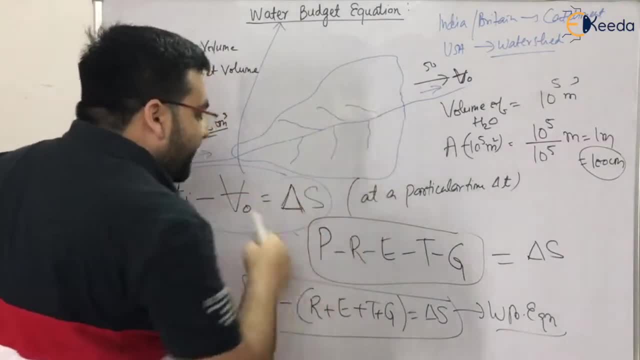 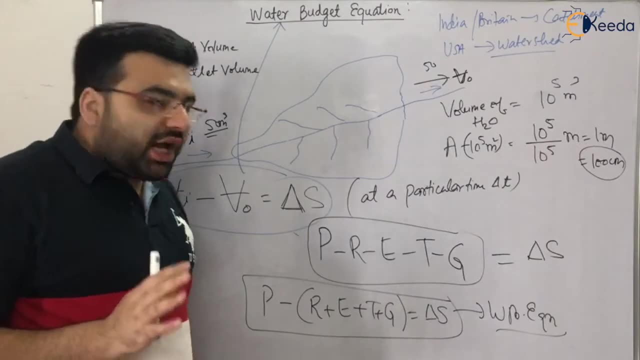 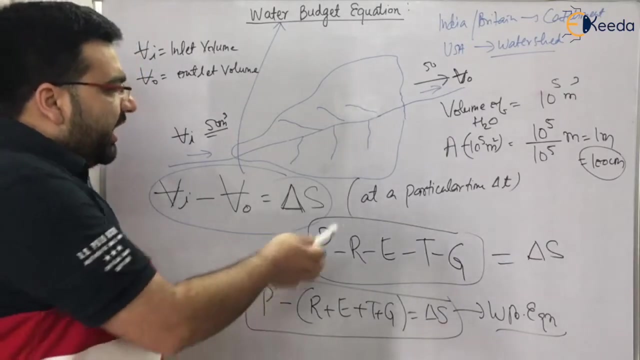 catchment area. so what is water we are left with? we are left with P minus. this thing is equal to storage, change in storage. simple now. I hope that you have understood the concept behind the water budget equation. okay, now, even if you have not understood, let me make you understand by. 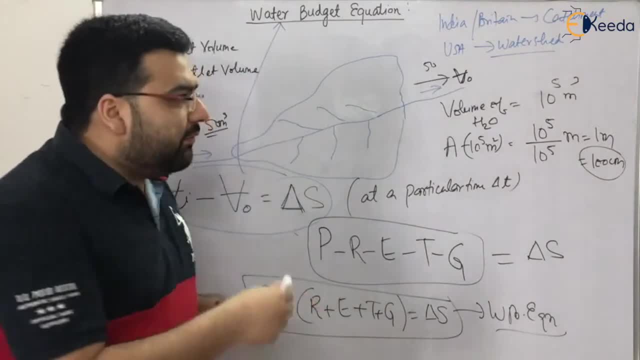 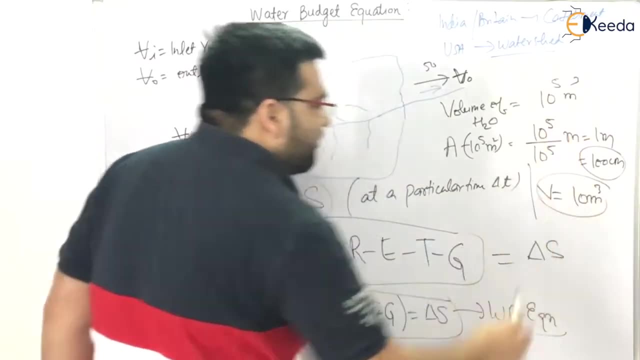 your very simple example. let us see that then you have a bucket and the volume of bucket is, let us say, 10 meter cube. it's a very big bucket. that's, the volume of the bucket is 10 meter cube. okay, you have put your bucket, let us say, under. 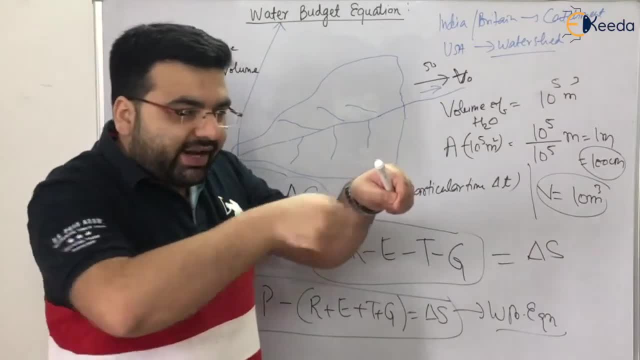 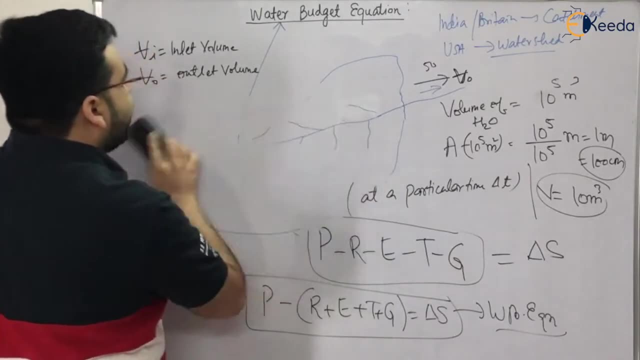 the Sun. you have put your bucket under Sun and you have also made one hole in the bucket. now let me draw it also. now, to make you understand a very simple term, let me also draw it. I hope you are getting right now. let us say that I have. 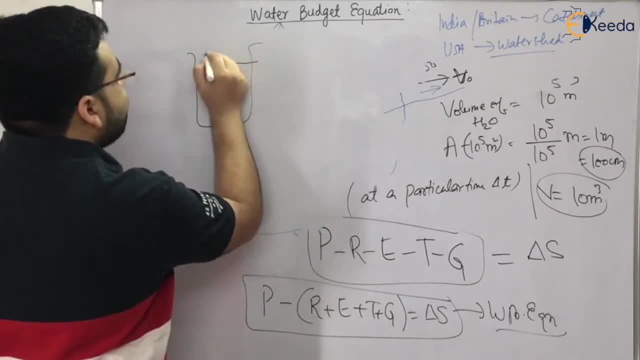 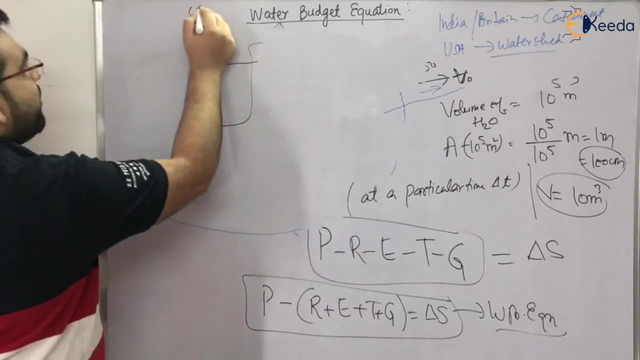 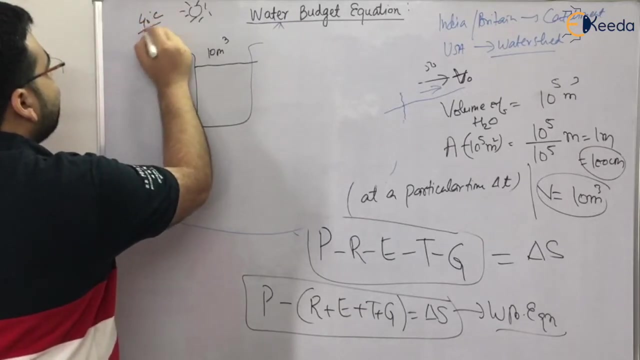 a bucket. the volume of the bucket is 1 meter. 10 meter cube. let us say it is a very big bucket, 10 meter cube. okay, now I have put it under the Sun. okay, under the sun rays. okay, the temperature is 40 degree Celsius. let us say it is a 40. 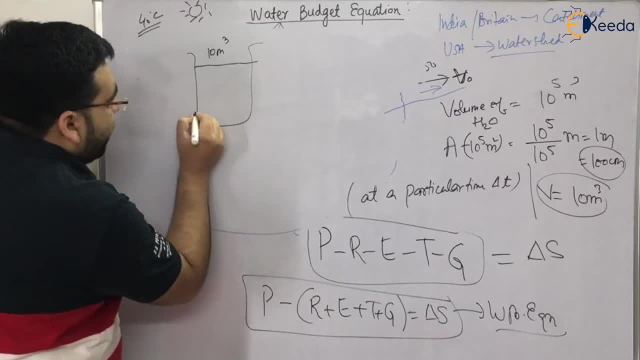 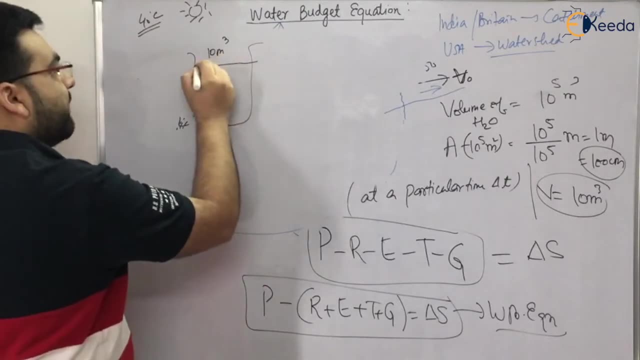 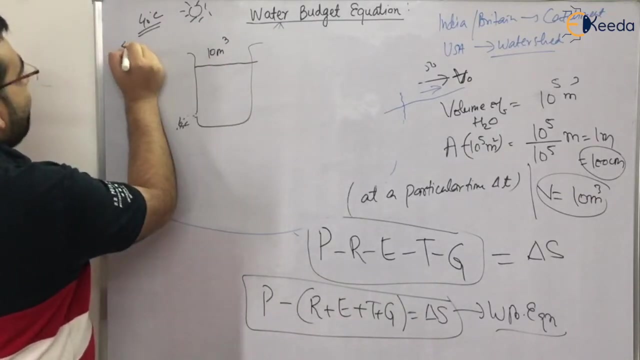 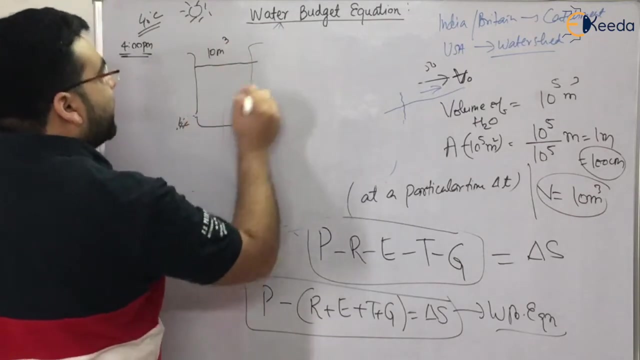 degree Celsius. yeah, now I have also made a hole here, which is continuously there is some outward discharge right, and initially I have filled the bucket up to its brim level, that is 10 meter cube. yeah, now, I started this experiment at 4 pm here now. I recorded the volume at 430 pm. 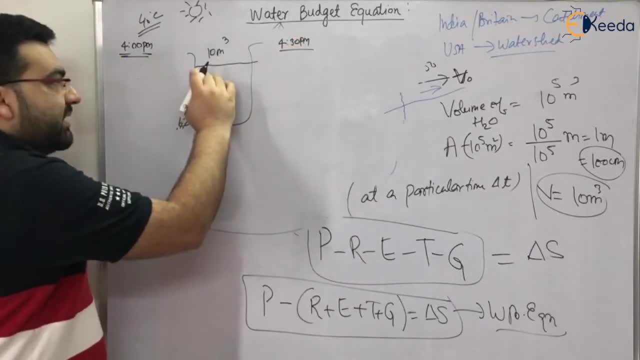 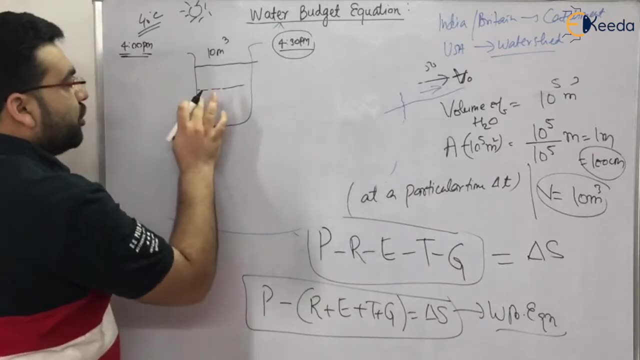 430 pm, 430 pm. so what will happen? there will be some declination up to here. now i will check the volume. how much is that volume? at 4 30 pm? how much is the volume? so you will say me that at 4: 30 pm the volume was. 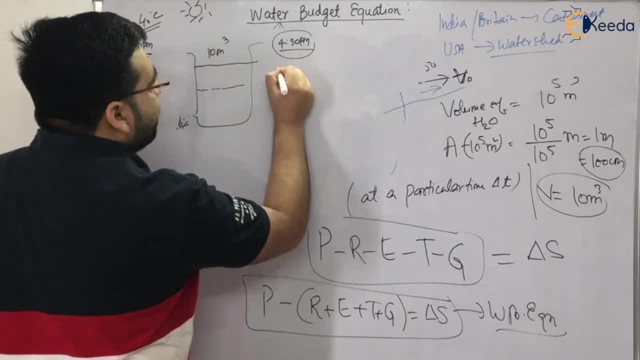 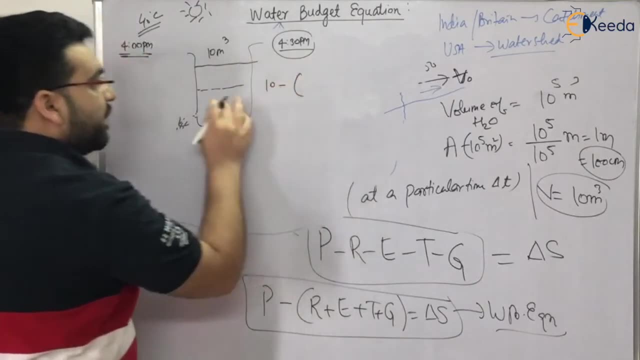 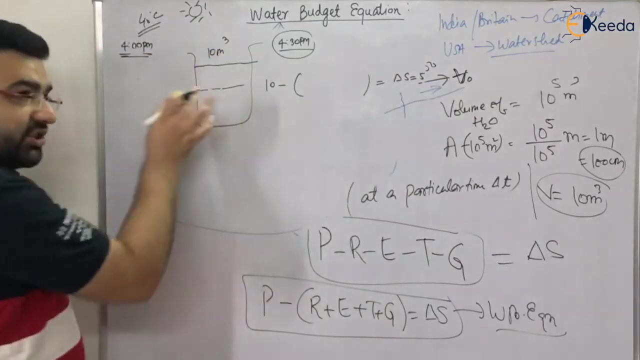 it is around. let us say: uh, five meter cube was left, so five meter cube is the initially 10 meter cube was the initial right now, minus now five meter cube is left right, so five meter cube is the delta storage. that is, five meter cube which is still left there right. how much has gone out? 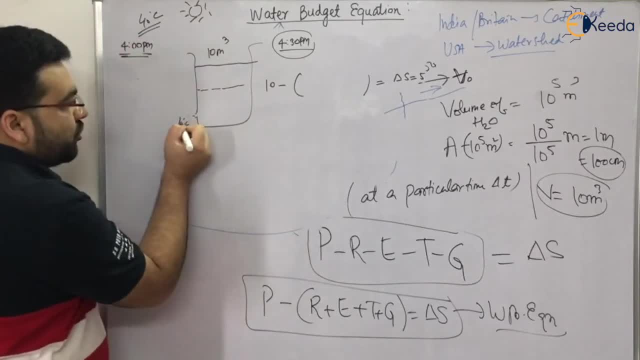 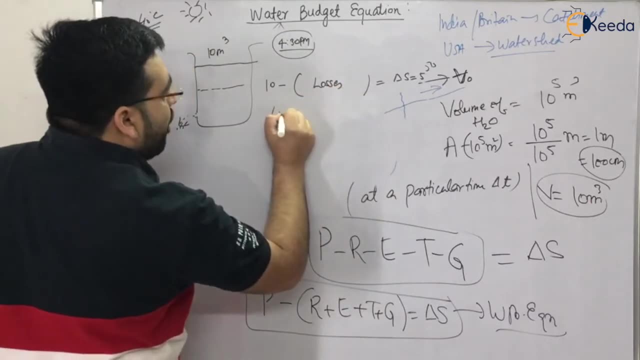 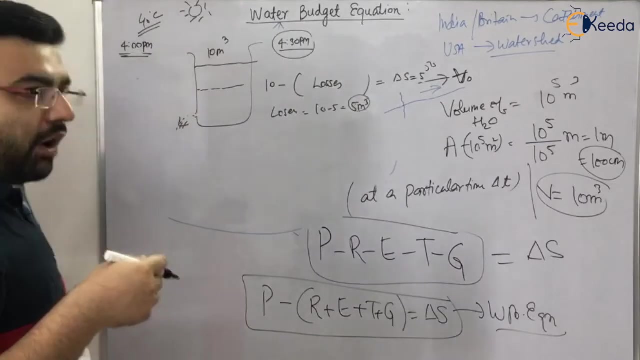 some will be evaporation, some has gone out from here. so i will say that this is your losses. are l losses? now i will calculate the losses, so losses will come out to be 10 minus 5 is equals to 5 meter cube. it means that 5 meter cube of water has- uh, you can say- left this bucket either by this: 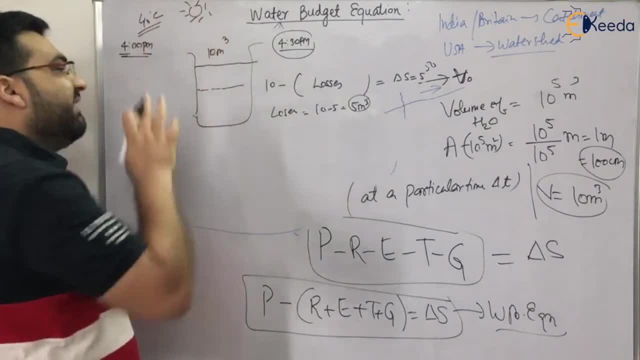 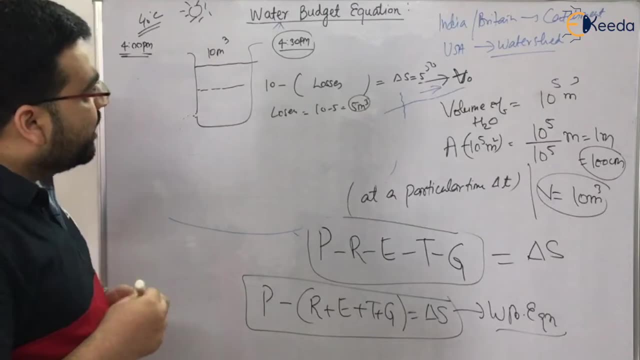 outward, you can say the hole, or by the evaporation. so this equation is known as the water budget equation. you have very simple experiment. i have just explained you in very simple terms that: take a bucket, make a hole right, put it. put the bucket, uh, under sun, let us say for one hour, for two hour. 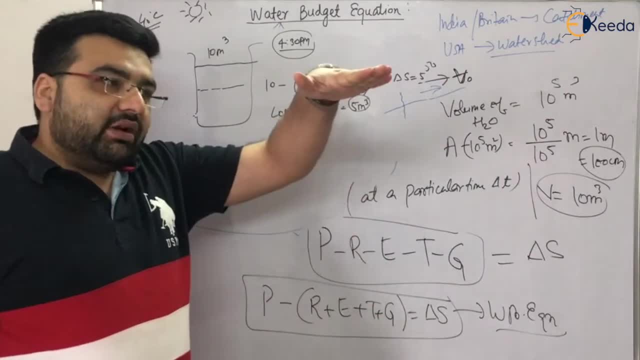 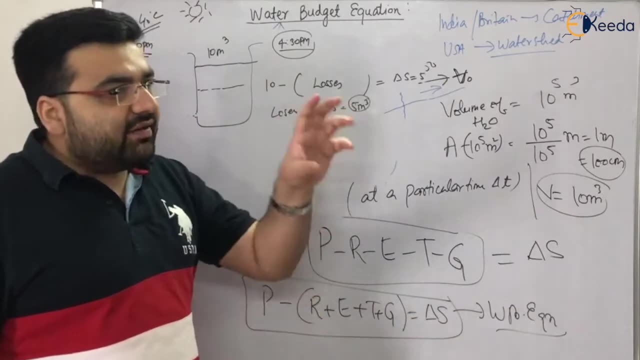 for three hour. after some time. what will be happening? there will be some declination on the water level. you will measure the discharge. you will measure the volume of the bucket, how much water is left in the bucket. that will be your delta is changing storage right and 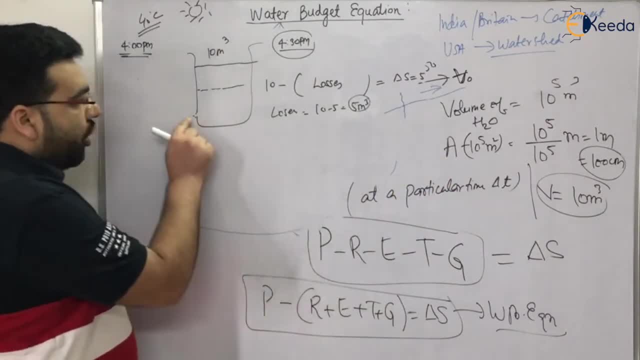 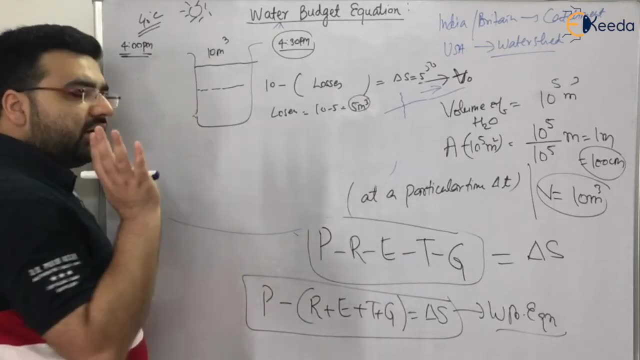 your losses will be. now. these losses will be in the terms of r- is the runoff which is coming out right evaporation. now there is no transmission because there are no plants and also we are not bothered about the ground material also. so your losses will be in the form of r plus. so this x. 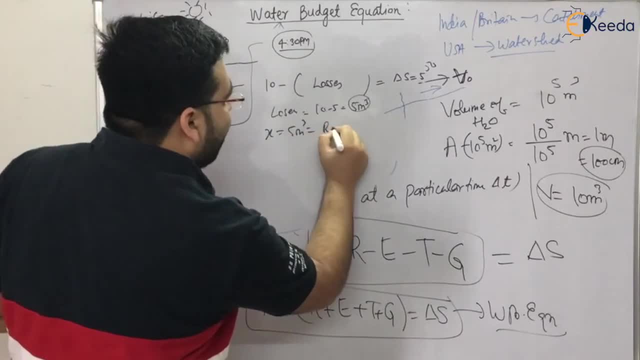 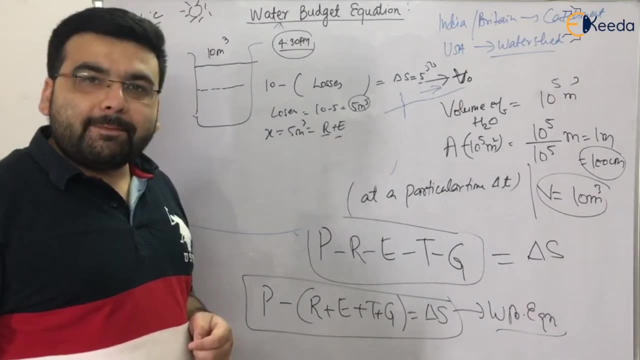 is equals to five meter cube. it will be in the form of r plus now, how much is r? how much easy they are. various form will termine r and e respectively. clear, okay, so i hope, students, that you have understood the water budget equation in a hydrologic cycle. clear.